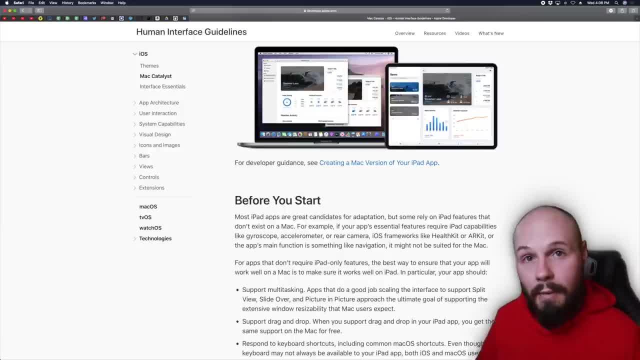 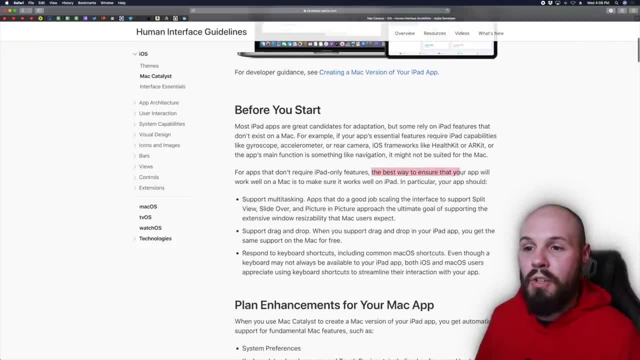 iOS apps to make sure they're still a great experience on the Mac. And we're not going to go through all these sections, you know, line by line. we're just gonna do a high level overview. But you know, basically, for Catalyst it says you know the best way to ensure that your app. 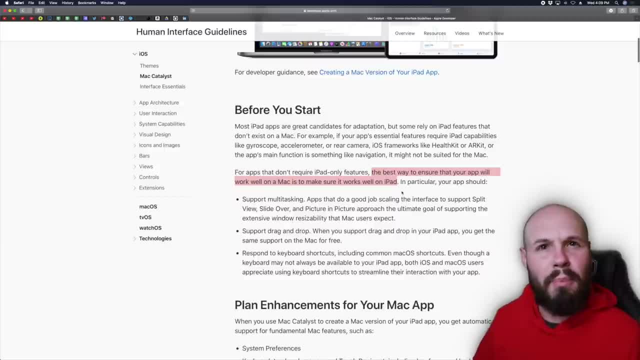 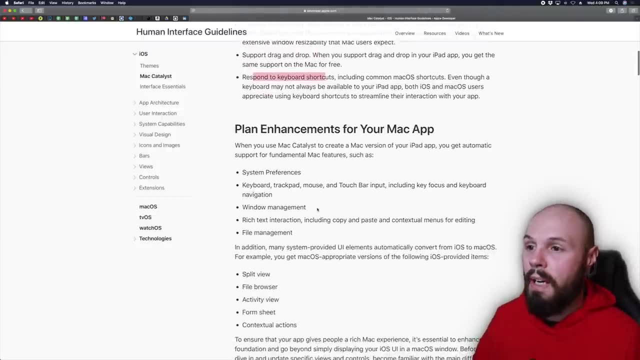 will work well on a Mac is to make sure it works well on an iPad. And then it gives you some particular things to look at: right Support, multitasking support, drag and drop onto keyboard shortcuts. it's going to give you all kinds of enhancements that you get for free. 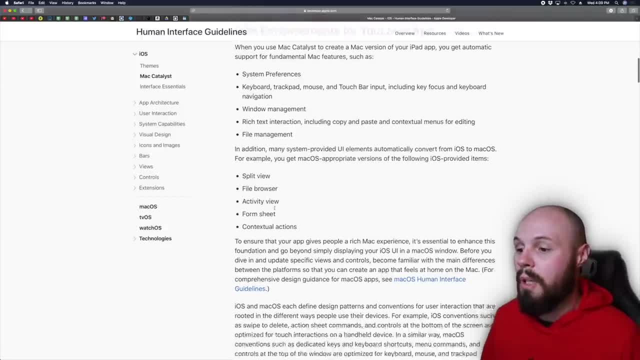 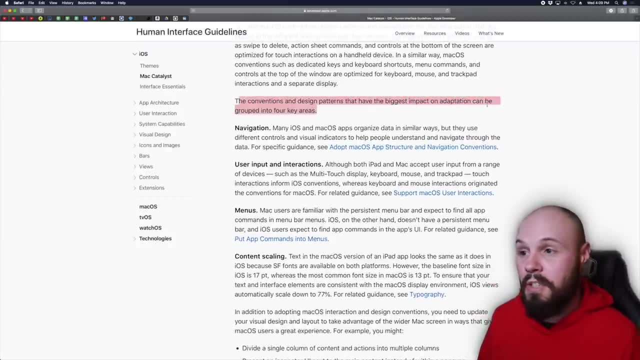 with a Mac app right System preferences keyboard, all that stuff split view. One thing I wanted to point out is that you should pay attention to. you know, the conventions and design patterns that have the biggest impact on adaptation can be grouped into four key areas. 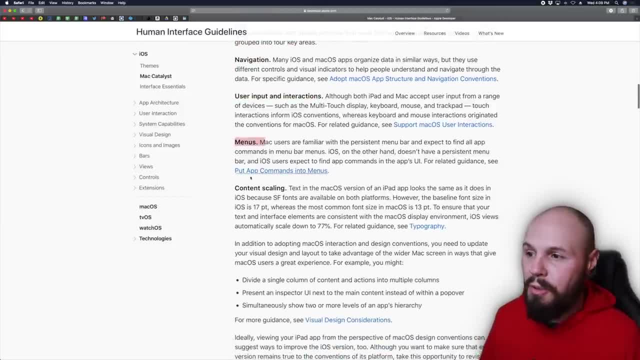 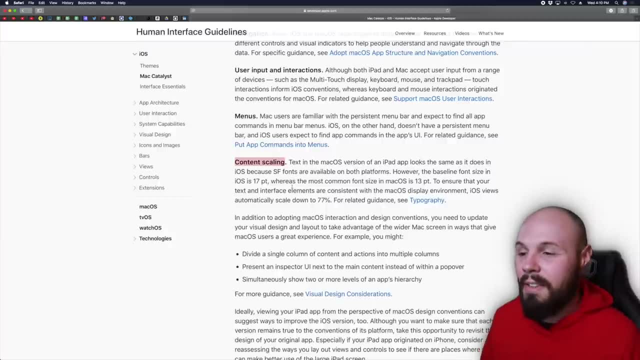 you know it talks about navigation, user input, interactions, how you should do- menus, the content scaling, obviously, like I'm looking at a 27 inch iMac screen, that's a lot different from an iPhone, So the scaling of the content is a big deal. So, basically, 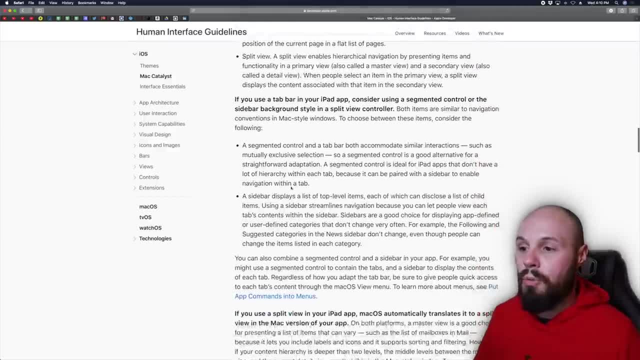 you know you're going to be able to do a lot of different things, So you're going to be able to do a lot of different things. So you're going to be able to do a lot of different things. So you're this is going to give you what you need to know to make your iPhone app conform to Catalyst And 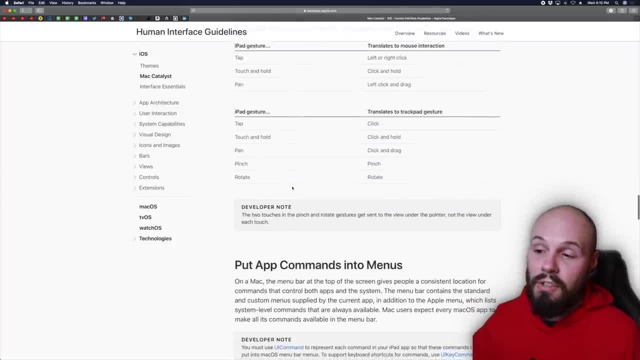 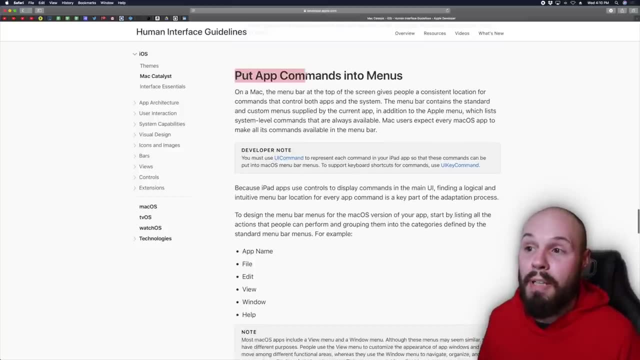 again, this isn't a Catalyst tutorial, but I'm scrolling kind of fast to show you kind of all the stuff that's in this. like there's so much information in the human interface guidelines, right, It's talking about putting your app commands into menus, right? You know when you're. 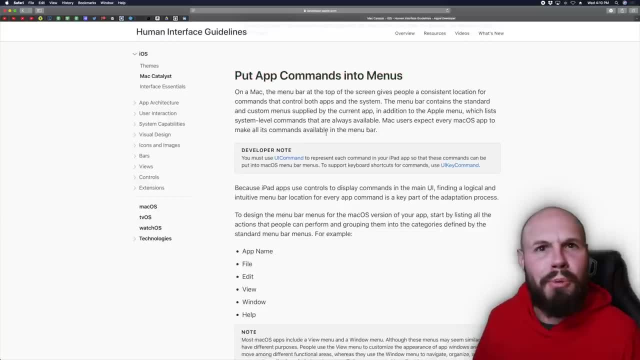 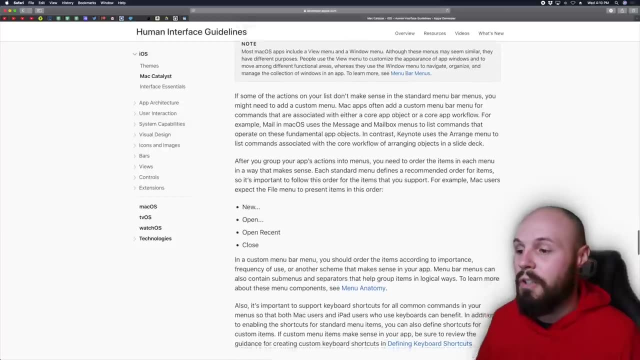 using your MacBook. you have the menu bar at the top there, And how do you, how do you convert your iOS stuff into that menu bar on the top of a Mac app? Well, this is going to tell you how to do that. So, again, this is the kind of information that is in the human interface guidelines, And 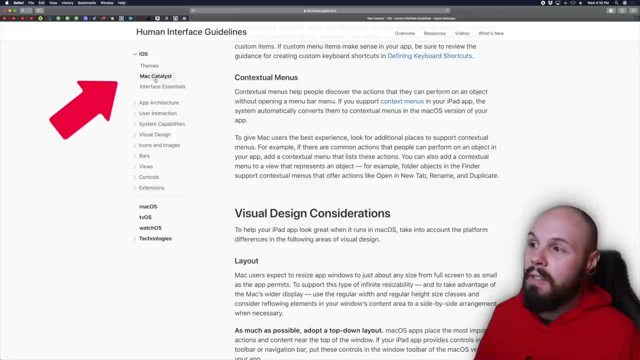 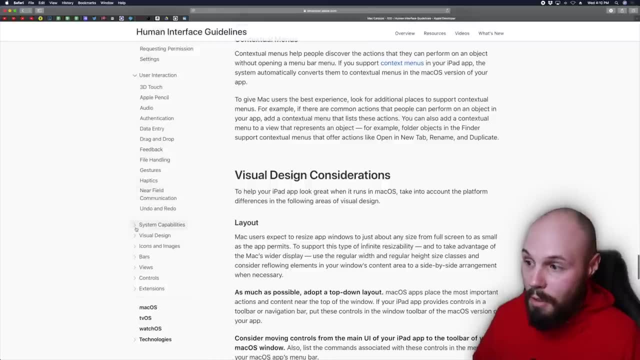 this is just one small section. If you look to the left here where Mac Catalyst, you can see like app architecture, you blow this out. Okay, now you get all these user interaction. look at all these user interaction system capabilities So you can see how in depth the human interface. 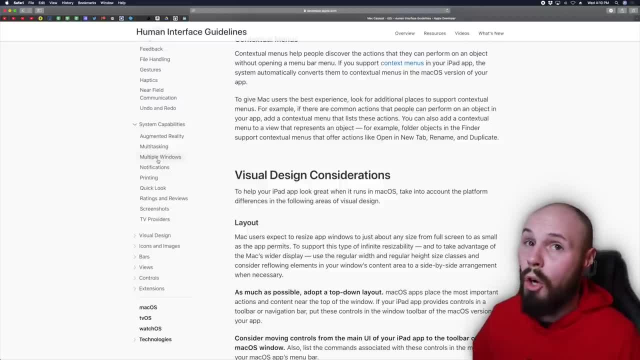 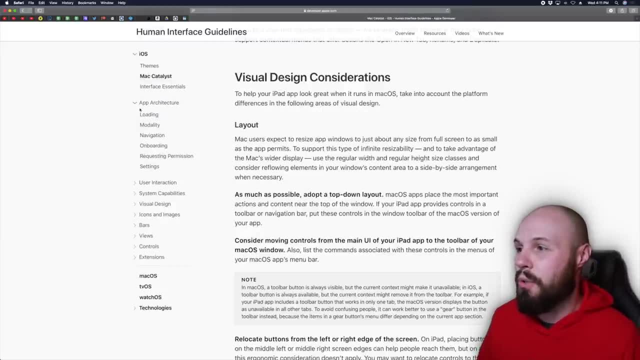 guidelines are- And we're only going to touch on just a couple topics- like it's a long read, But again, fundamental for iOS developers. So let's go back up real quick to a smaller section here, just to show you an app architecture, like even the mundane stuff like loading, like this: 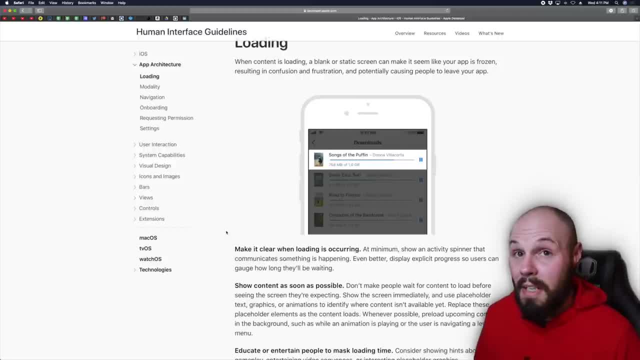 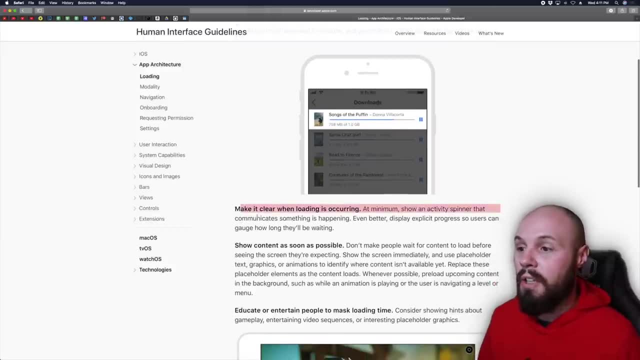 tells you how to properly handle your loading states for your app. So, like I said, it gets into like the nitty gritty. This isn't just high level big picture stuff, Like again you want to make it clear when when loading is occurring. 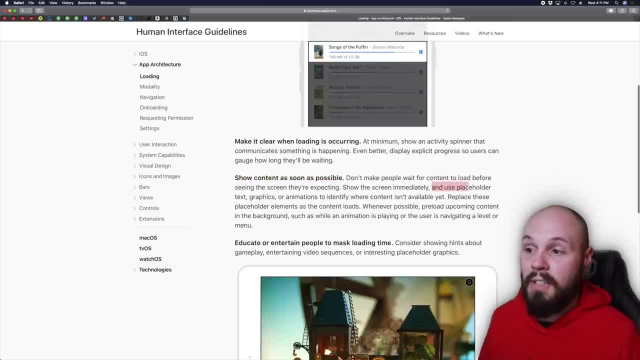 show content as soon as possible. You know. it says you know, use placeholder text, graphics, animations to identify when content is available and then replace those placeholder images when you know when content is there. may seem common sense to some people, But again for junior. 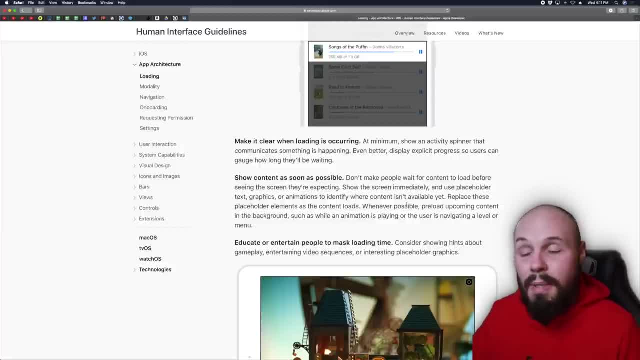 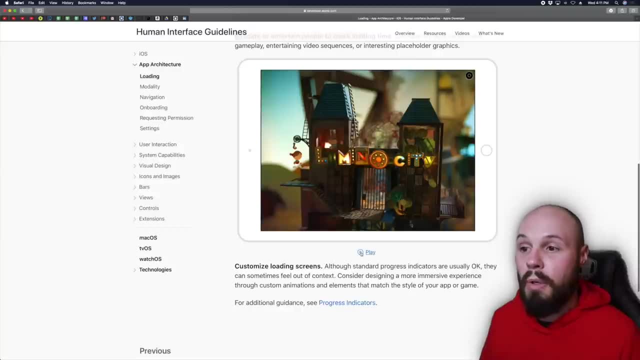 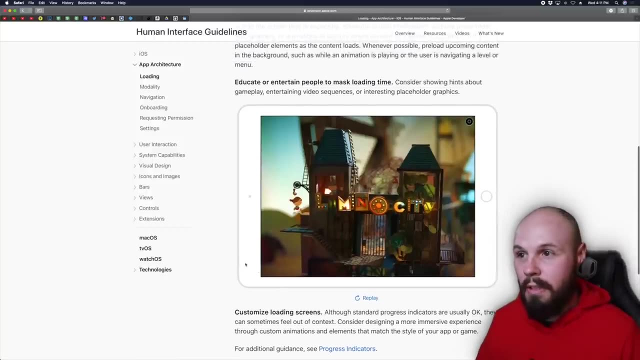 developers or people that are aspiring to be iOS developers. you know this may not be common knowledge to you. Educate or entertain people, while you know to understand what's going on. So, again, this is just an example of some of the stuff you're going to get. 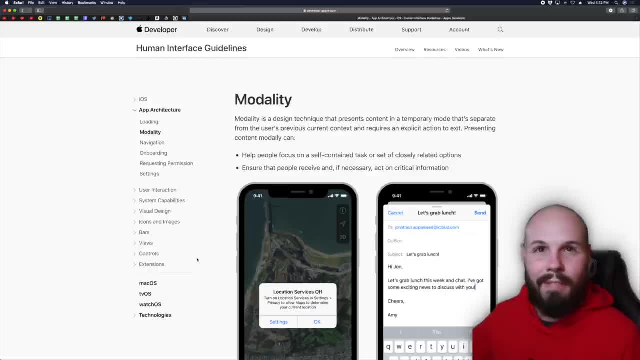 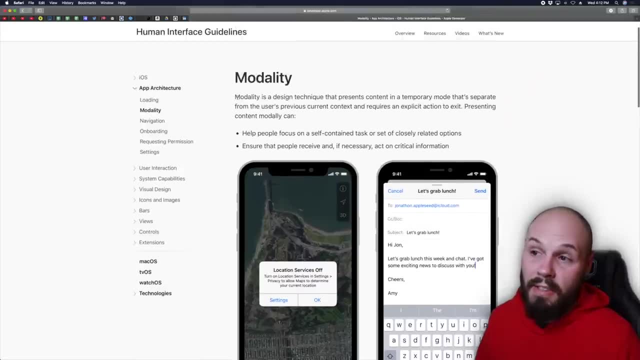 moving on to the next example, Let's talk about modality, And I'm just kind of going down the list again, just showing you what this is like. you know, a modal screen is these screens, that kind of slide up from the bottom. It says modality is a design technique that presents content in a 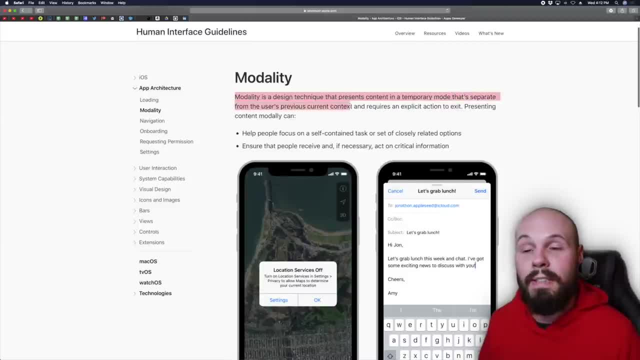 temporary mode that's separate from the user's previous screen. So if you're using a modality, you don't want to use it in the previous current context. That is the key there. It's a it's like a separate action from what the user's current context is And it talks about when you should. 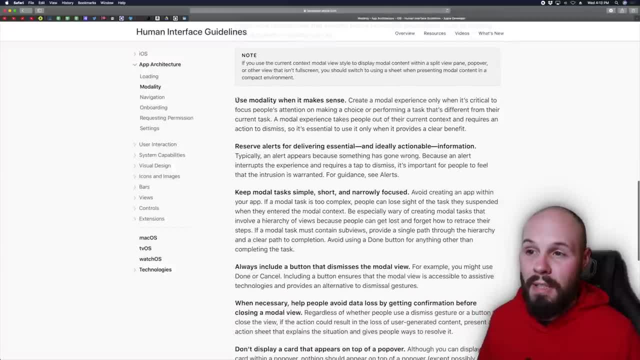 use modals the best way to use them, you know. use modality when it makes sense. create a modal experience only when it's critical to focus people's attentions on making a choice or performing a task that's different from their current task. That's kind of what I just said. 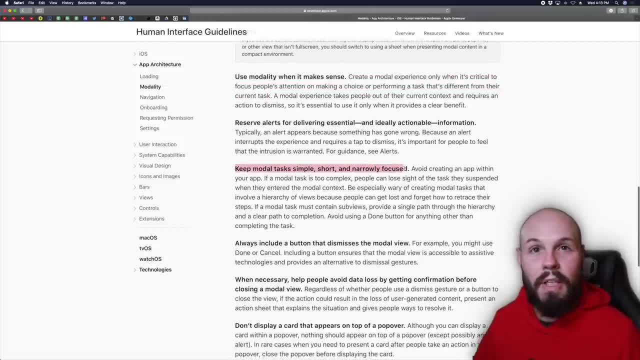 You know you want to keep the modal tasks short and simple and narrowly focused, right, You don't want to avoid having an app within your app. So again, there's just best practices for UI UX. If you're not strong in like just user experiences or UI, just reading the human interface guidelines. 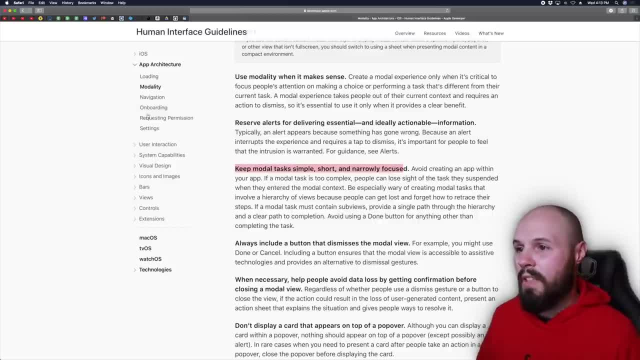 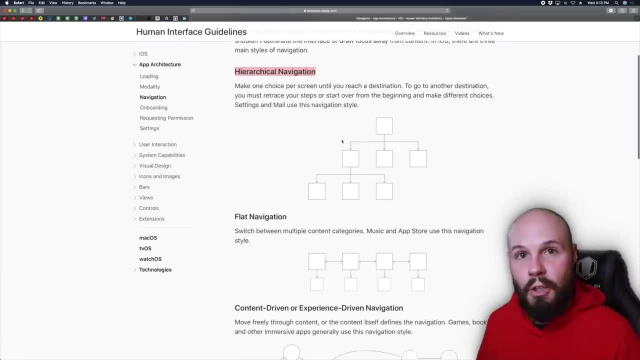 will up your game a lot. And then more fundamentals like navigation right. This will teach you the different types of navigation right: Hierarchical navigation, where you know you go down this tree here and then to go back. you got to kind of retrace your steps back to this top screen. 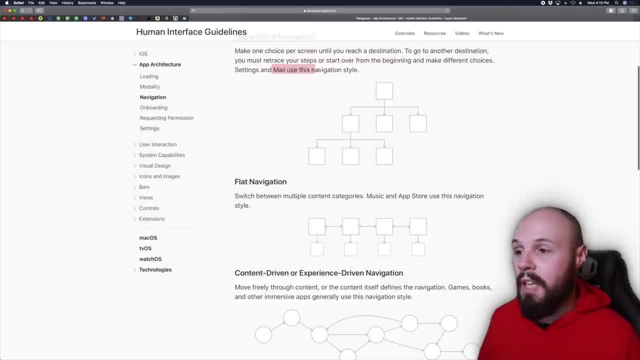 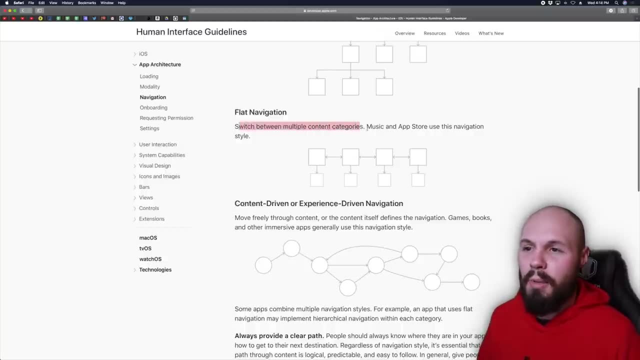 or you know, and it gives the example of like settings or mail, use this navigation style. you know understanding the flat navigation style. switch between multiple content categories. this is usually kind of like a tab bar. you know the music. 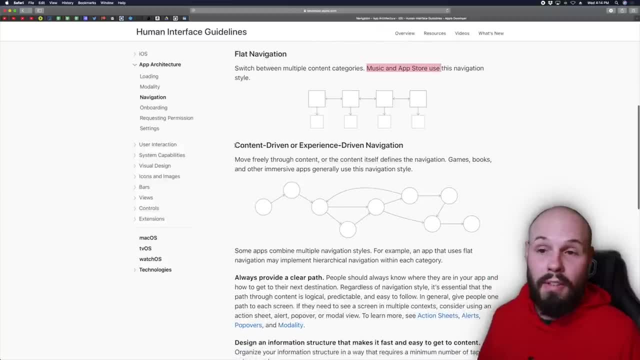 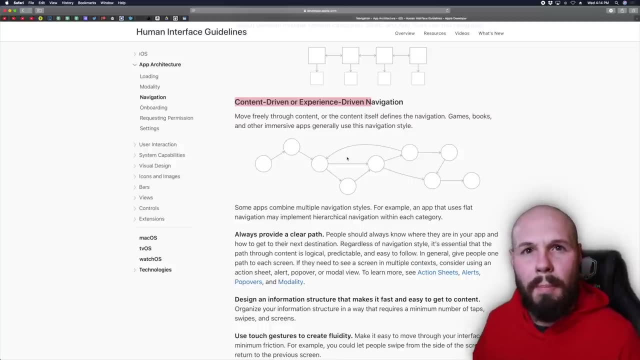 and the App Store uses navigation style, then content driven navigation right, And you can kind of see and understand all the different navigation patterns. you know that an app can use and when to use the right one. And the last piece I want to point out here because I know a lot of. 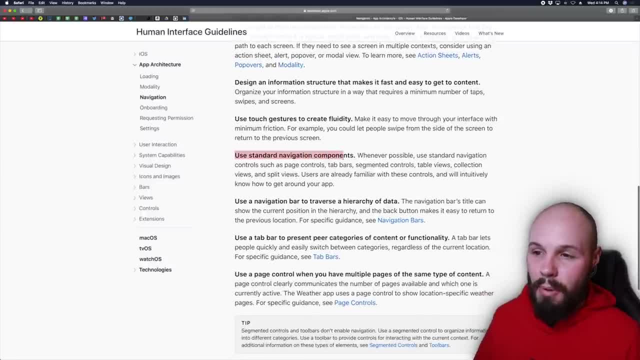 people try to reinvent the wheel. here is: use standard navigation components you know whenever possible, right? Because, like I said, users are already familiar with these controls and will intuitively know how to get around your app. This is kind of the full circle I went through as a 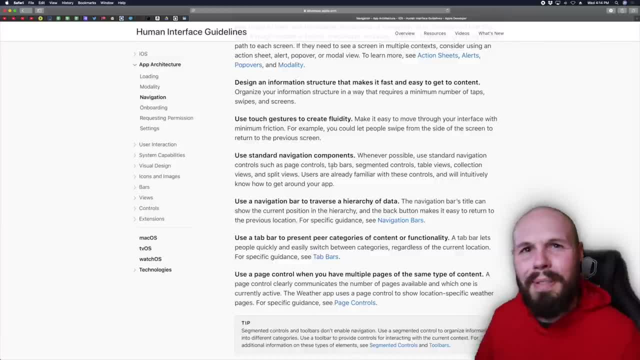 developer. Like when I first started, I was like: No, I want to be unique, I want to be different- default stuff. And then you quickly learn that like, yeah, you may feel cool to do that, But your users aren't going to know how to use your app, So keep it simple, use the default stuff when 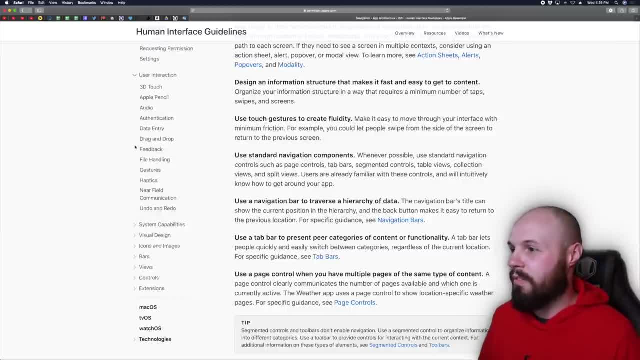 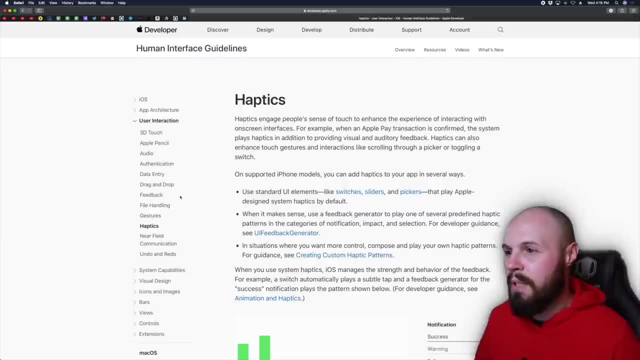 applicable And then two more topics. Like I said, I just want to give you a breadth of different fields. here we're gonna talk about haptics, because haptics is kind of unique and interesting And I think they're underused in a lot of apps. I mean, Apple uses them a lot, But basically, 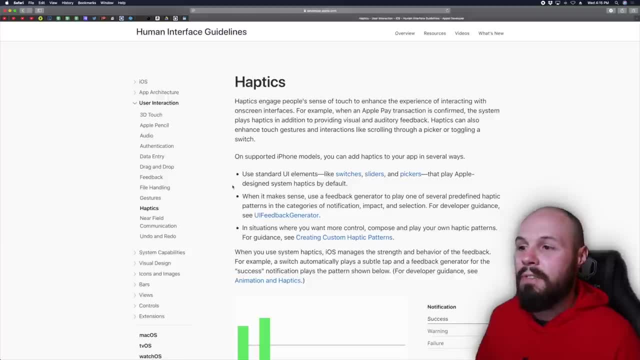 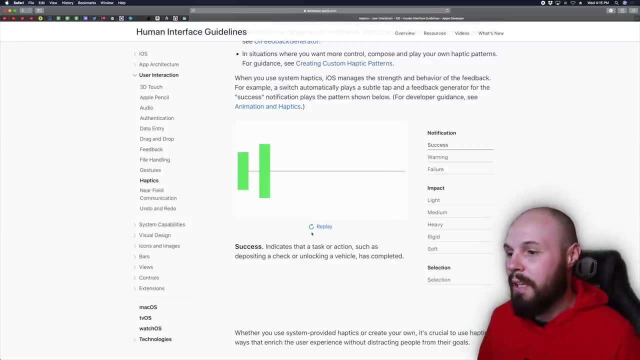 haptics is that little tap tap on your phone that you feel And this kind of tells you how to use it, when to use it, some advice, you can kind of get an example of it. You can't hear that, But that that plays like a little sound And it tells you some tips on like 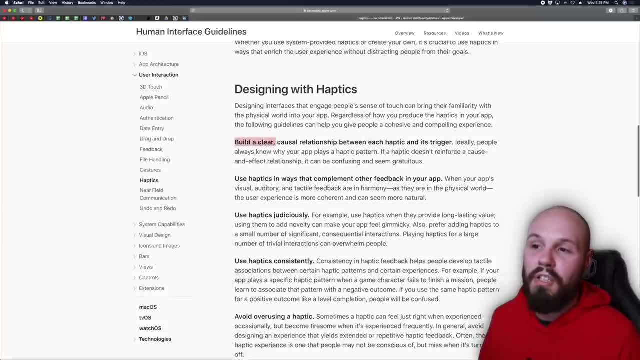 designing with haptics. I, like this, build a clear and casual relationship between each haptic and its trigger. Ideally, people always know why your app plays a haptic pattern. If a haptic doesn't reinforce a cause and effect relationship, it can become confusing and seem gratuitous. 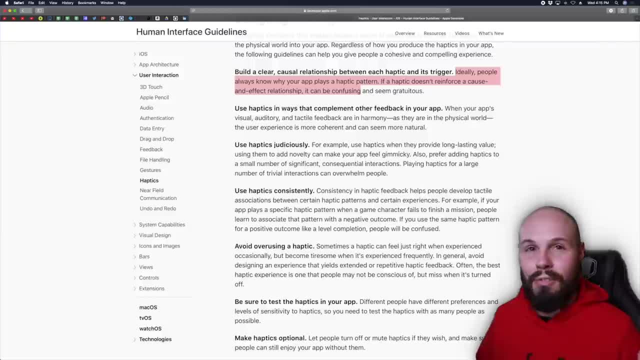 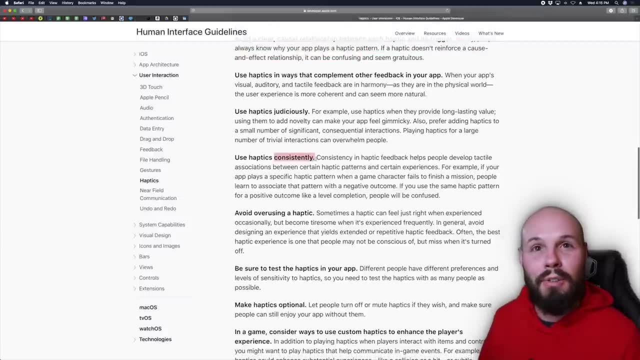 And then things like you know, just don't overuse haptics, Don't use haptics for every little thing, right? Just like too much of a good thing, Never good right. And just be consistent with it, right. If you have a haptic for a success sound. 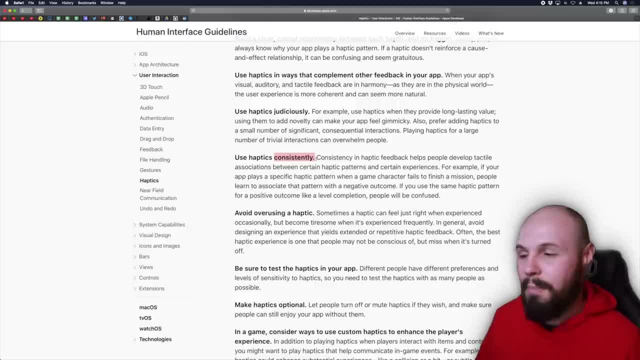 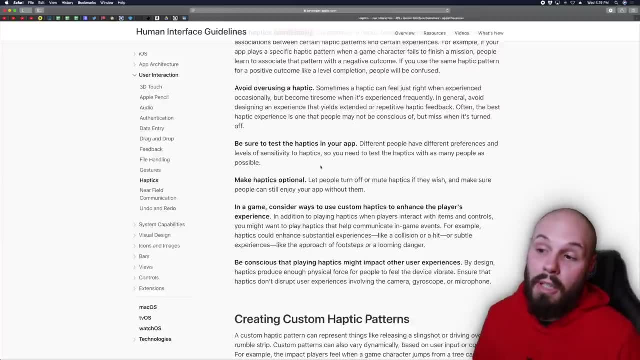 event. don't have the same haptic for the failure event, right? Just be consistent with it. And again, as you can see, more just information on how to properly use haptics in your app And then even tells you like, if you want to create your own custom haptics, here you go. 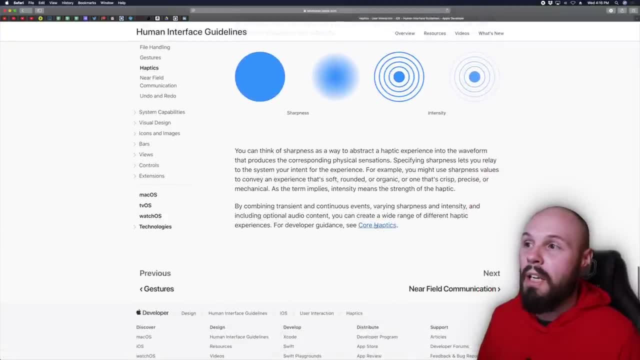 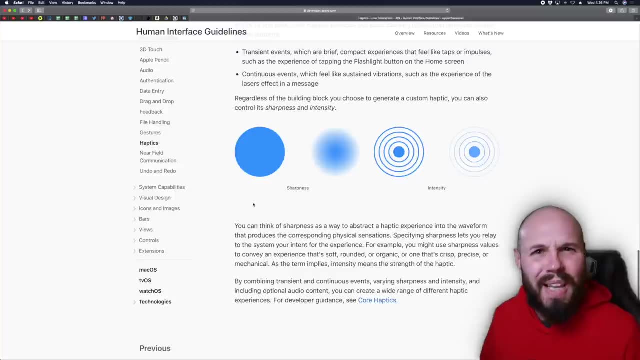 it tells you all about. you know the proper way to use it, even links to the core haptics documentation here for you to dive deeper. you know as the developer, but again, something as kind of niche as haptics, right? Not a lot of people use them. 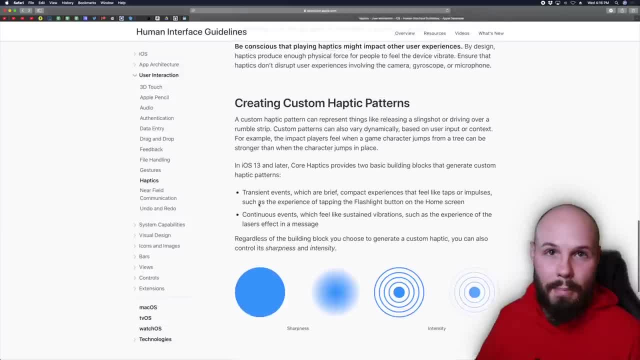 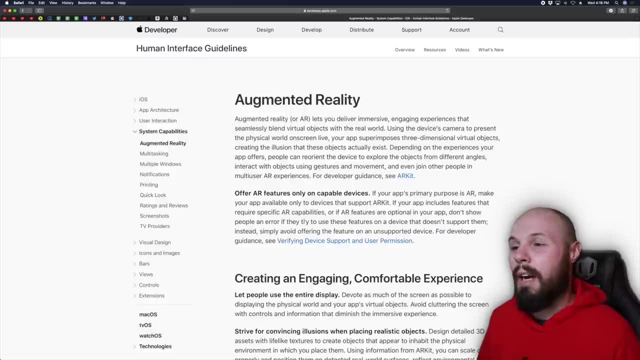 you're getting a lot of information on how to properly use them within your app. And then, lastly, we're really going to skim over this one because it's augmented reality. Obviously, that's going to be a big deal. You've heard about the glasses coming out. 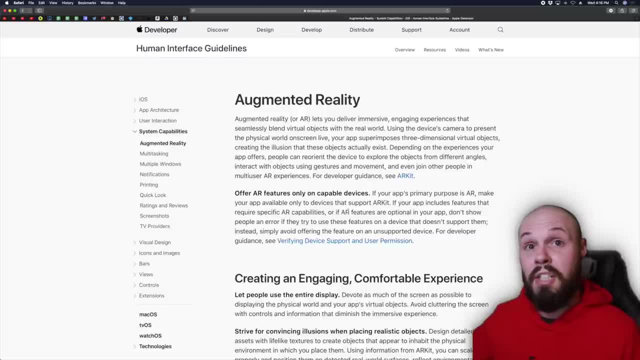 Apple's really stressing it. The reason I say we're going to skim over this is because this section is really really long, basically outlines like how to build a proper AR experience, So we're going to kind of skim over it very quickly. Again, I highly encourage you to come here.